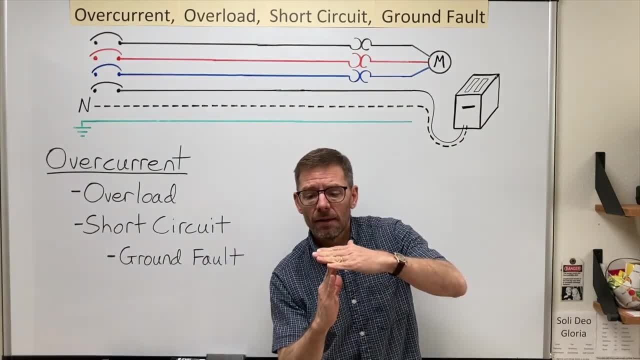 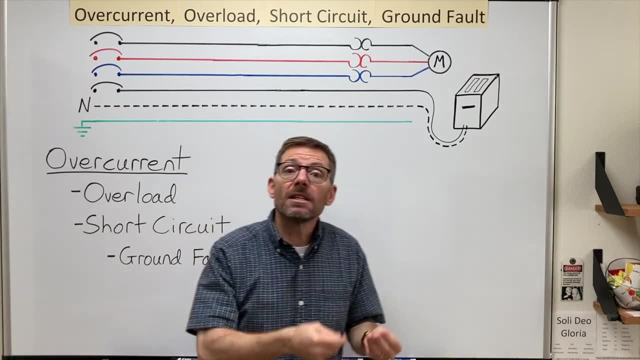 Well, that's going to be too many loads. After a little while that breaker is gonna trip. We have an overloaded circuit, Or I could have a piece of equipment drawing too much current. Perhaps I've got a motor that I'm working too hard and I gotta ease up on it. 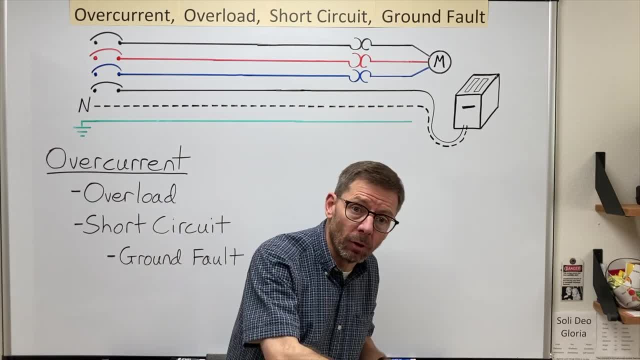 Or sometimes if we have too high of a load, we can bump it up about 15 Fahrenheit, you right, Like just laying out 15- GirET, putting the most pressure on it is like there should voltage, too low of a voltage, depending on the type of equipment that can result. 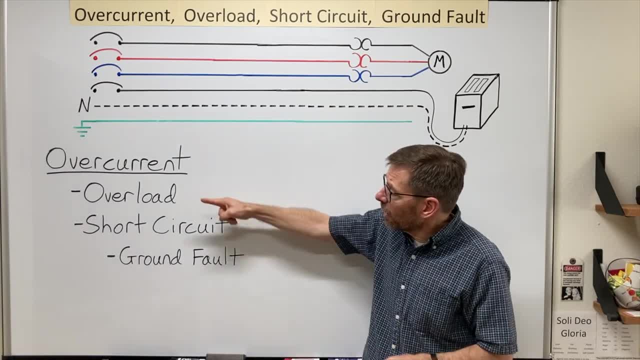 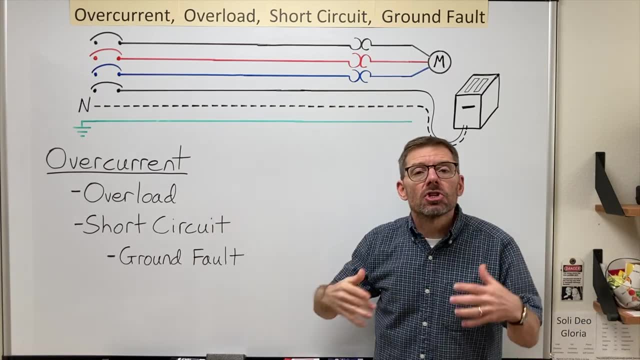 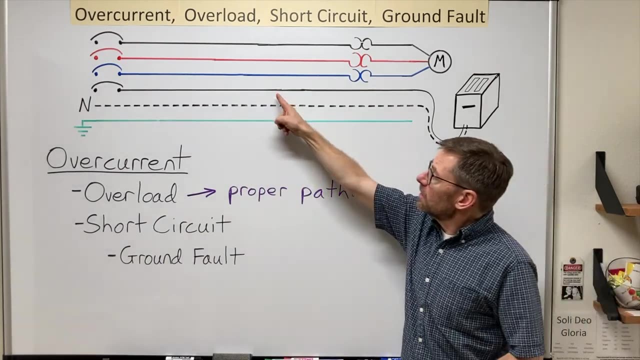 in too much current flow as well. But one thing I want to say about overloads is that the current is flowing in the proper pathway. there's just too much of it. By proper pathway I mean that the current is going down the hot through. 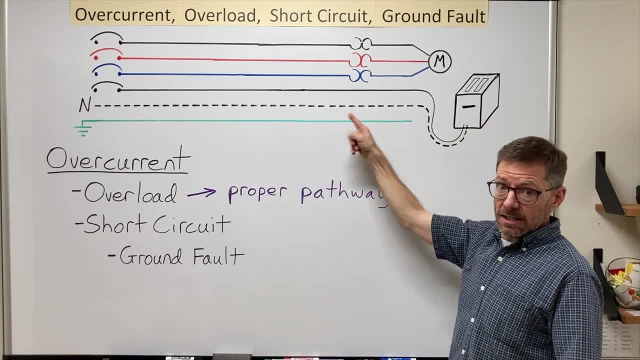 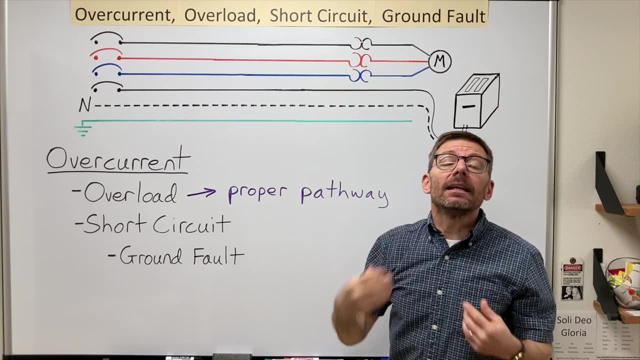 the load and back, the neutral, back and forward, It is AC or in a multi-phase situation, it's going back and forward on the appropriate conductors in the intended way. Now this definition goes on to tell me that if the excess current 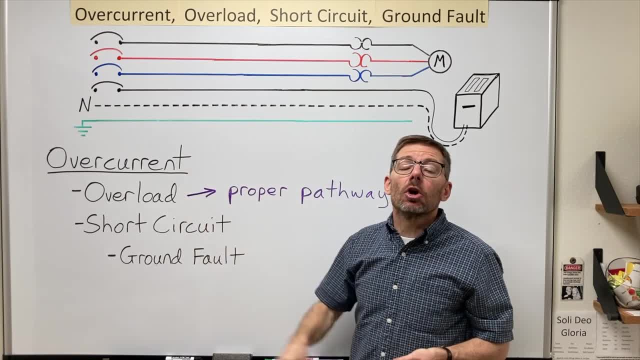 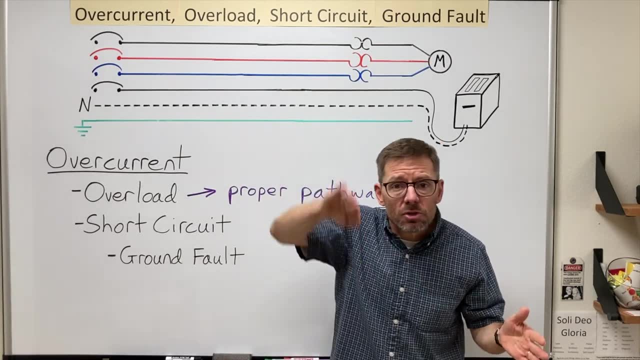 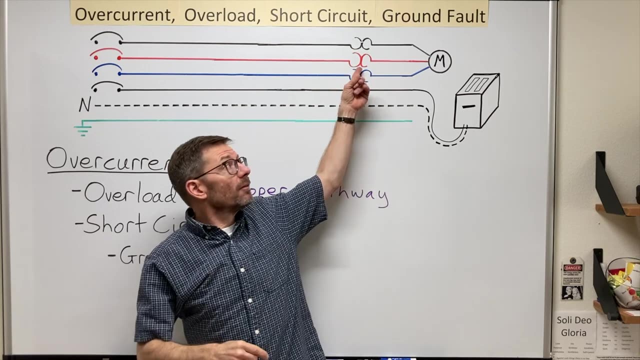 continues for too long, it can cause damage or dangerous overheating. But there are safe overloads, ones that last just a few seconds, even a few minutes or something sometimes longer, depending on the intended characteristics of the devices involved. 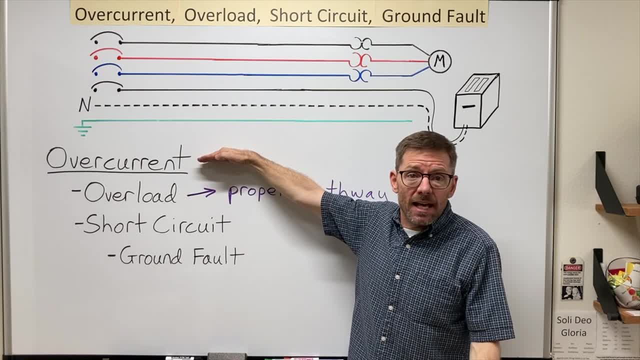 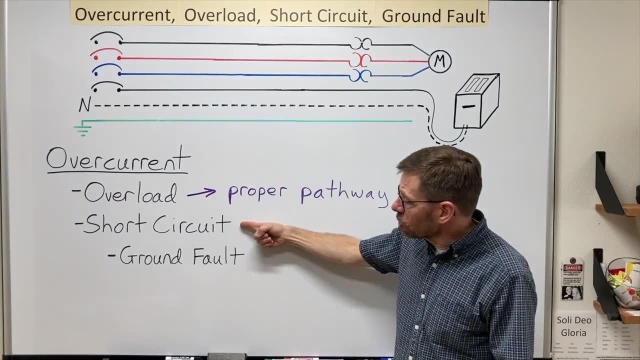 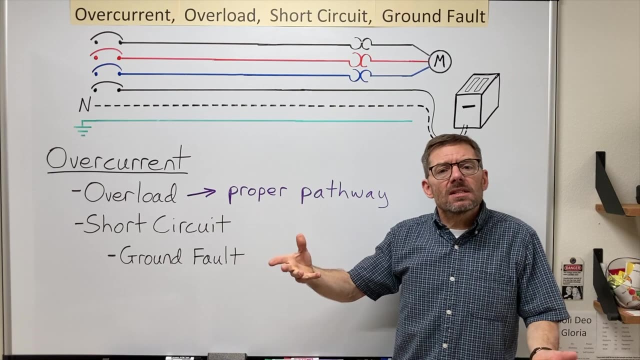 And there's an info note under this definition that addresses that issue. But the final sentence under overload says that a fault such as a short circuit or a ground fault is not an overload. So what's the main distinction between overload and these faults? 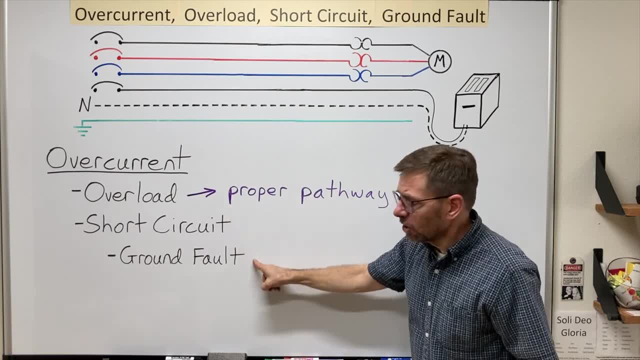 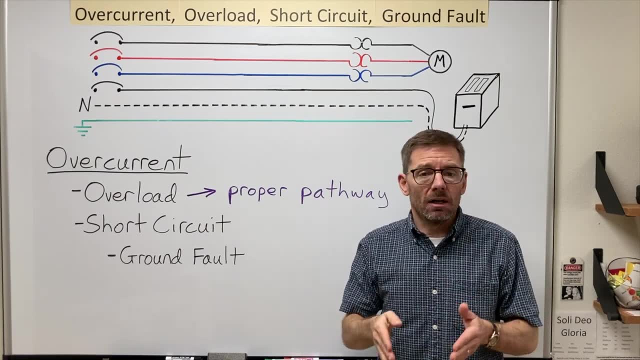 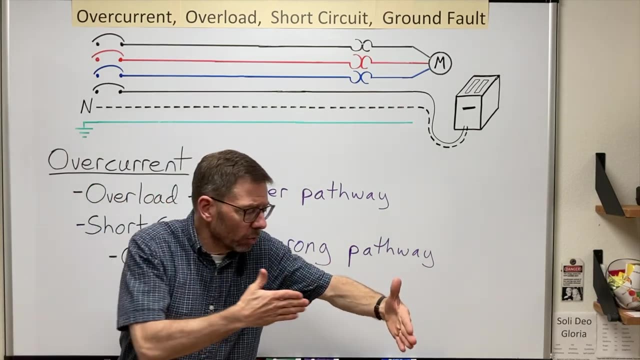 Well, I'm going to say that these fault currents are not flowing in the intended pathway. they're flowing in a wrong pathway. Here the current is taking a shortcut. Think of driving down the road and instead of going all the way down to the light and waiting to turn right, 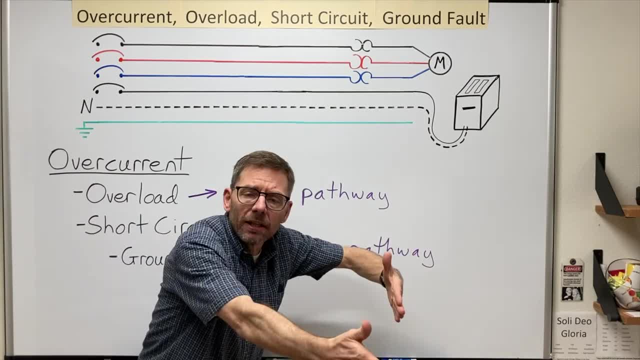 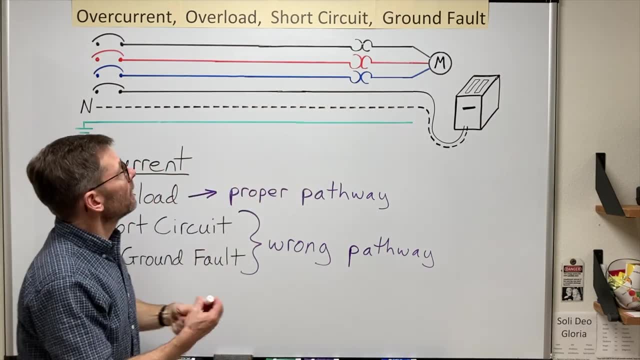 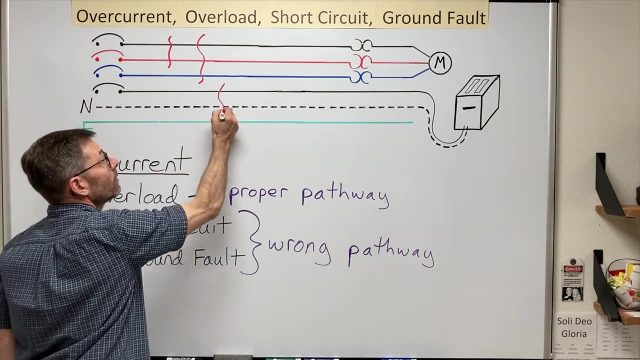 you just decide: nah, I'm going to cut through the gas station or the parking lot, whatever's there. The current is doing the same thing. Instead of going Through the load and back, it's just taking a shortcut. It can be a line-to-line, or maybe line-to-line-to-line in a three-phase system, or line-to-neutral. 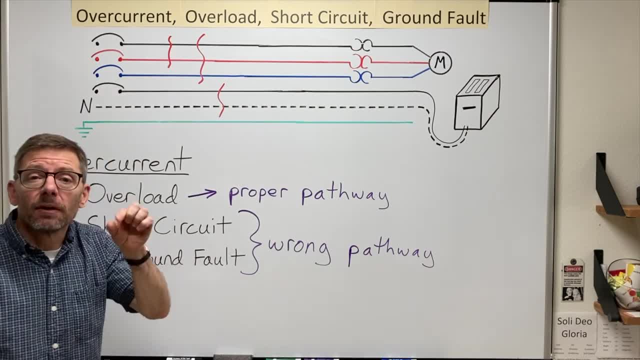 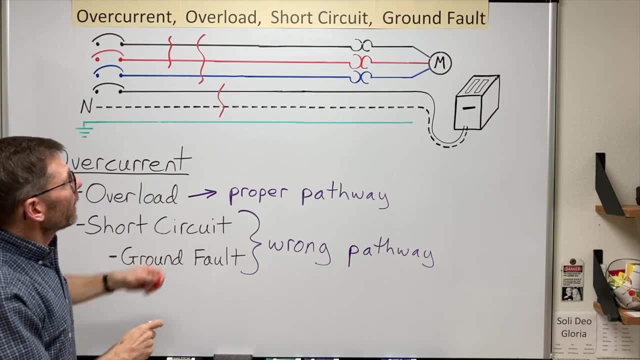 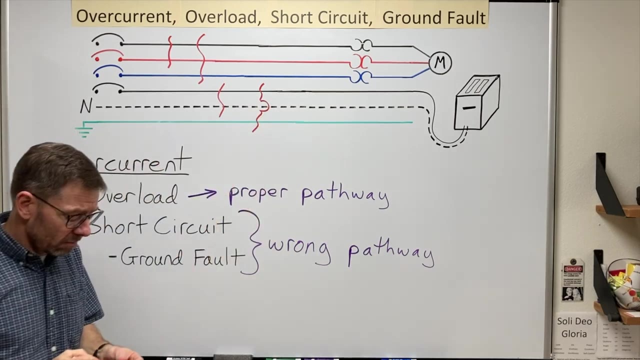 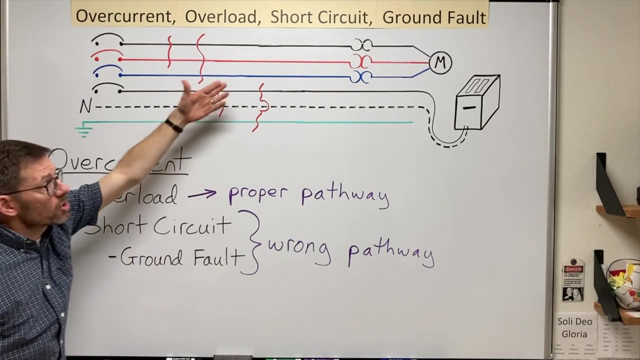 And how much resistance would there be there? Often there's very little resistance and therefore, how much current Loads of current. Now we could also have a hot To the ground. Now, whenever the ground falls, The ground is involved, we call it a ground fault. so it's still a short circuit, still taking the wrong pathway. 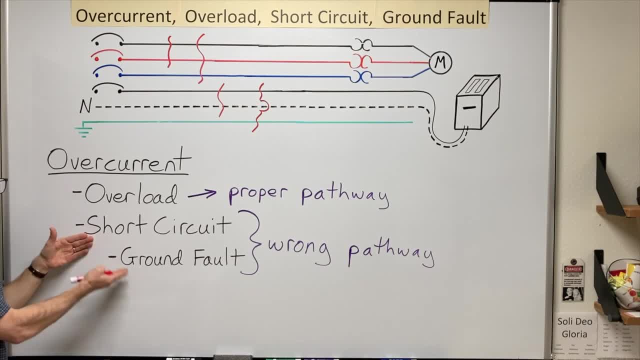 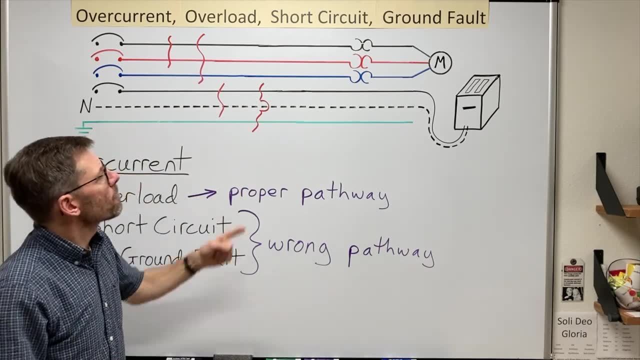 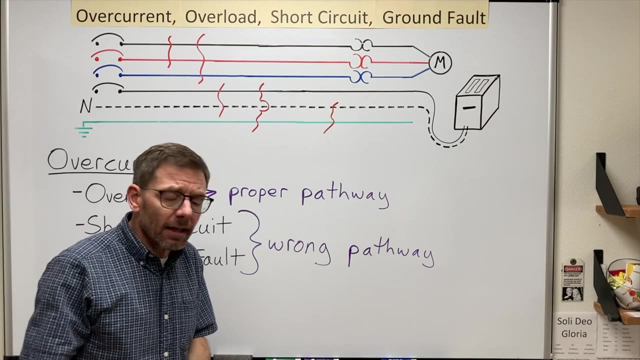 so you'll often see ground fault as a sub-category of short circuit, and a lot of current can flow there as well. We want that device to open right away. But then could we also have a neutral-to-ground? Yeah, that'll open a ground fault device. but if you look at the definition for ground fault, 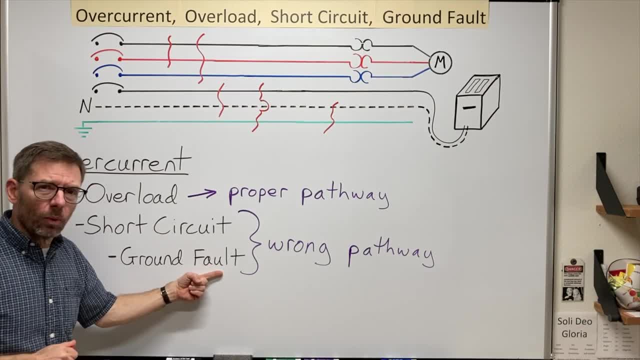 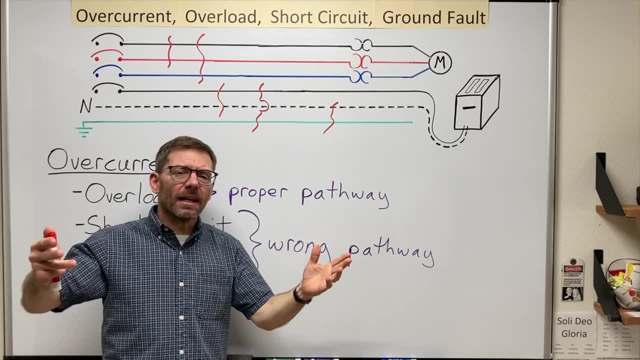 Yeah, that'll open a ground fault device. but if you look at the definition for ground fault it says that it is an unintentional pathway between the hot and the ground. When I first read that I was confused. I said: wait a minute, why not neutral-to-ground? 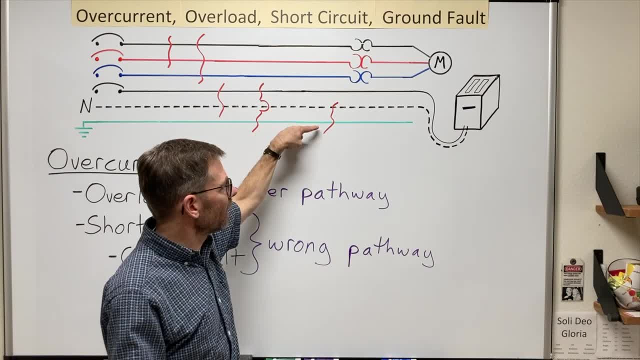 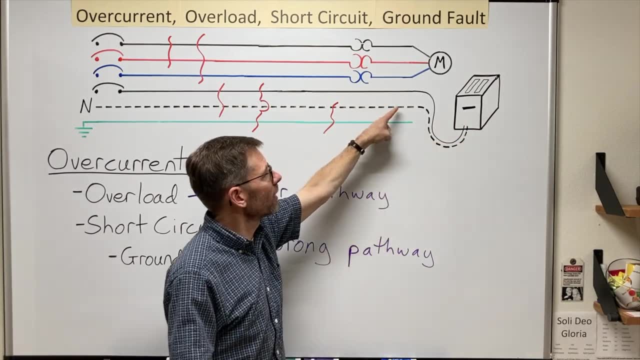 But then I thought about it: Is this hot connected to this ground? Is there pathway? Yes, Through the load there is pathway. It is electrically connected to the ground And although this fault may not cause an excess in the ground, 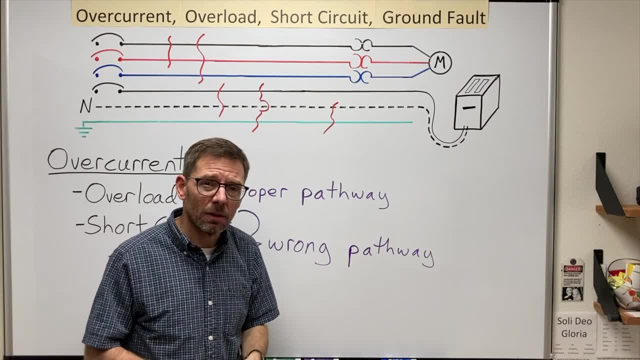 And although this fault may not cause an excess in the ground, and although this fault may not cause an excess of current to flow, and although this fault may not cause an excess of current to flow, it causes current to flow in a potentially dangerous pathway. 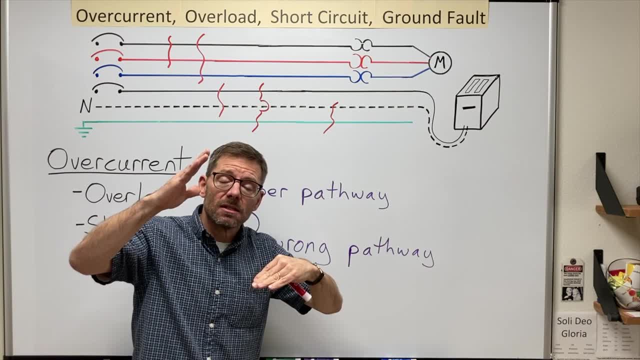 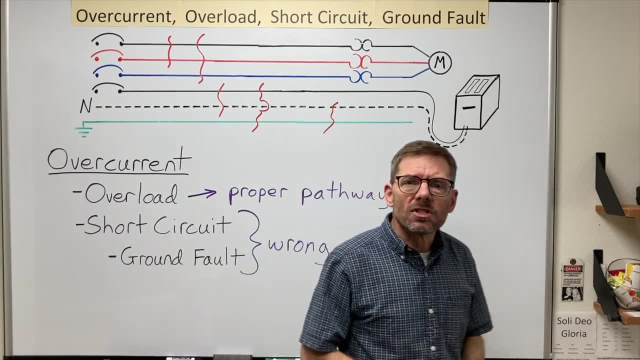 so it will open the ground fault device and stop the circuit from operating. So what are the main differences, then, between my overloads and these short circuits? So what are the main differences, then, between my overloads and these short circuits?